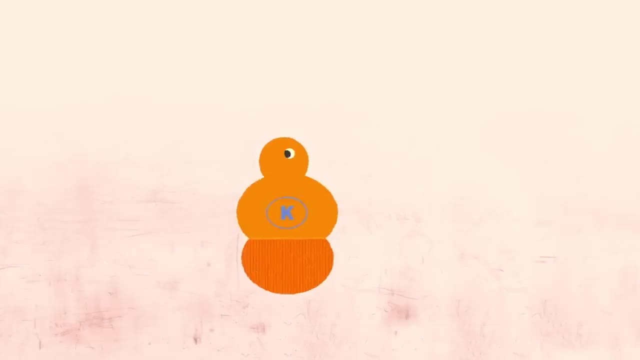 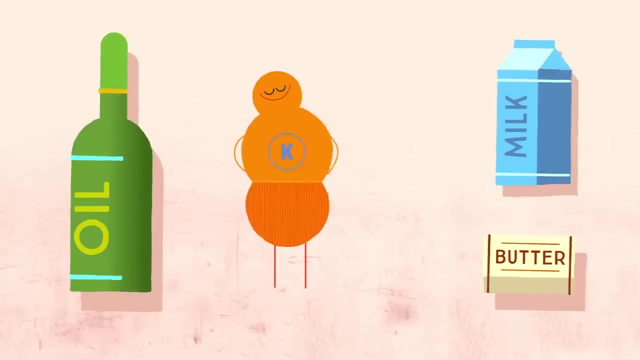 and can move around freely within the body. For lipid-soluble vitamins, dissolved in fat and found in foods like dairy butter and oils, this trip into the blood is a little more adventurous. These vitamins make it through the stomach and the intestine. 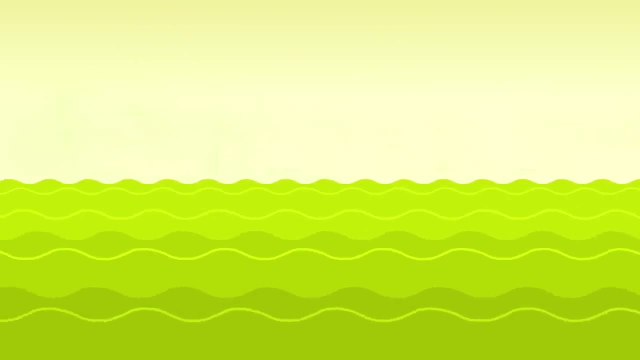 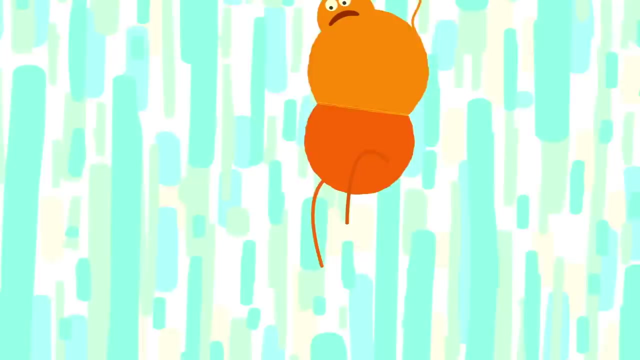 where an acidic substance called bile flows in from the liver, breaking up the fat and preparing it for absorption through the intestinal wall. Because fat-soluble vitamins can't make use of the blood's watery nature, they need something else to move them around. 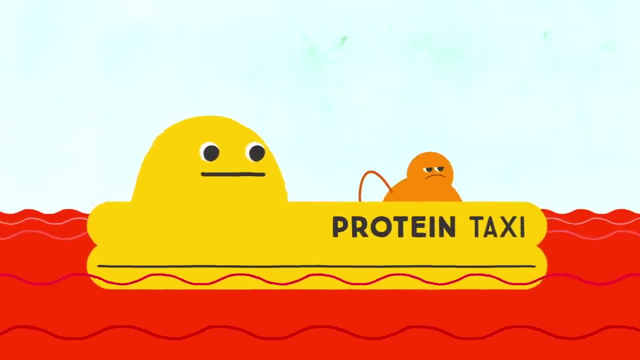 and that comes from proteins that attach to the vitamins and act like couriers transporting fat-soluble vitamins into the blood and around the body. So this is a little bit more complicated than you might think. So this is a little bit more complicated than you might think. 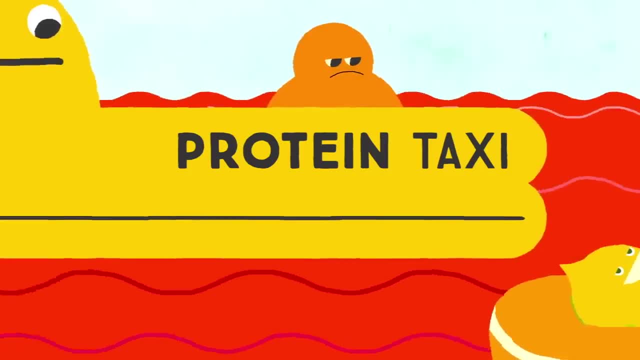 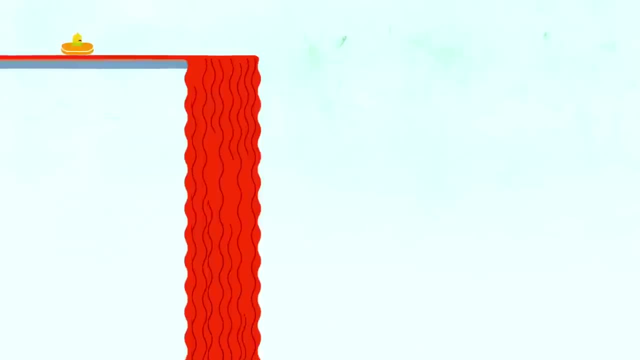 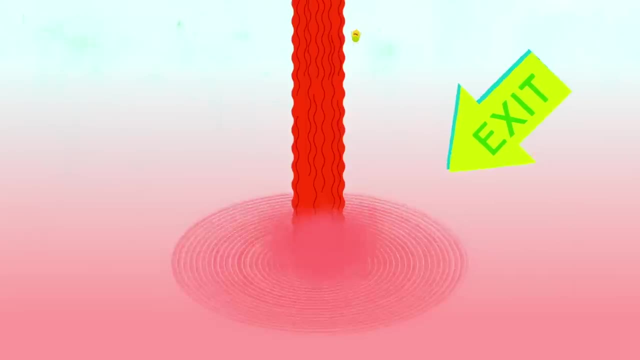 This difference between water or fat-soluble vitamins determines how they get into the blood, but also how they're stored or ejected from the body. The system's ability to circulate water-soluble vitamins in the bloodstream so easily means that most of them can be passed out equally easily via the kidneys. 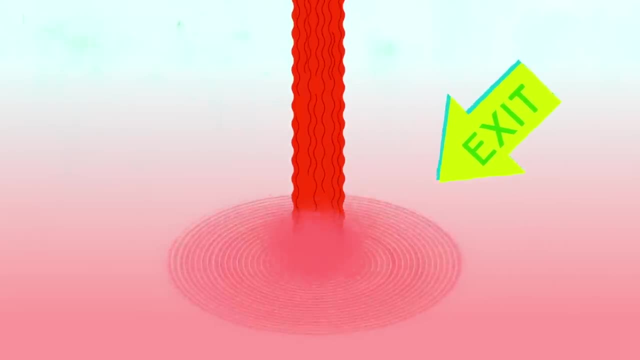 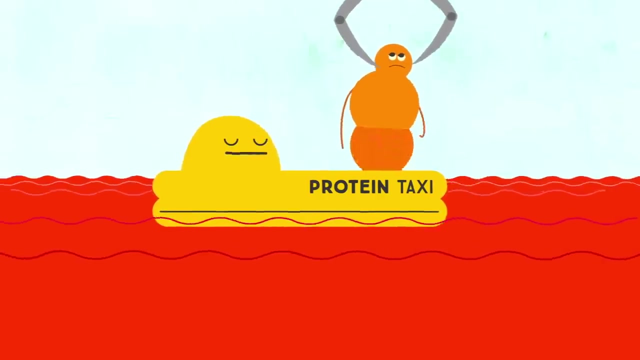 Because of that, most water-soluble vitamins need to be replenished on a daily basis through the food we eat. But fat-soluble vitamins have staying power because they can be packed into the liver and then in fat cells. The body treats these parts like a pantry. 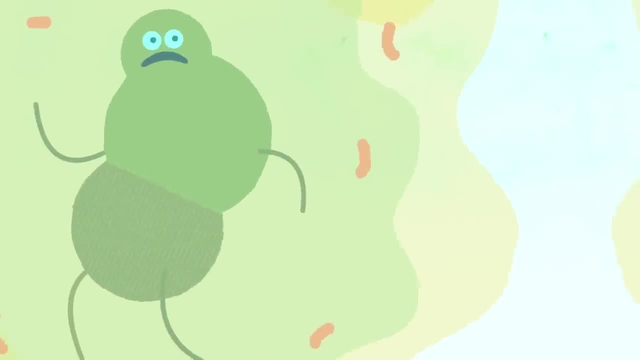 storing the vitamins there and rationing them out when needed, meaning we shouldn't overload on this type of vitamin, because the body is generally well-stocked. Once we've figured the logistics of transport and storage, the vitamins are left to do the work they came here to do in the first place. 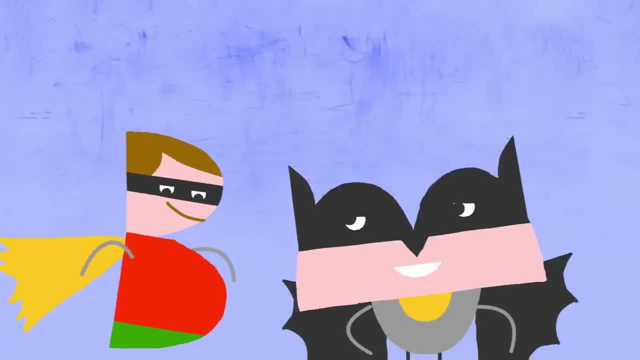 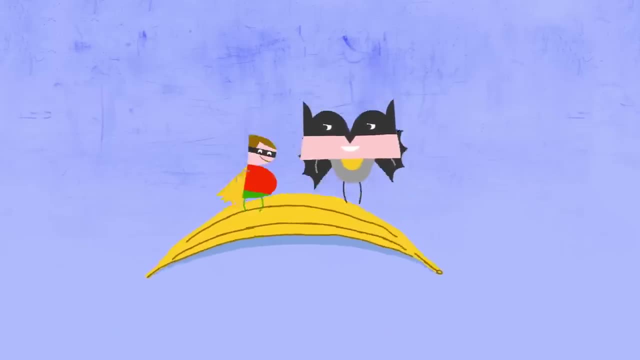 Some, like many of the B-complex vitamins, make up coenzymes whose job it is to help enzymes release the energy from food. Other B vitamins then help the body to use that energy. From vitamin C you get the ability to fight infection. 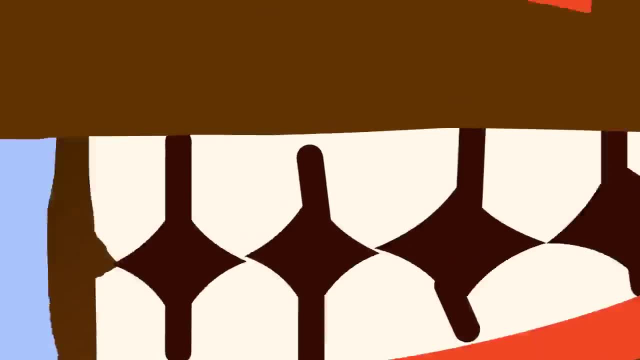 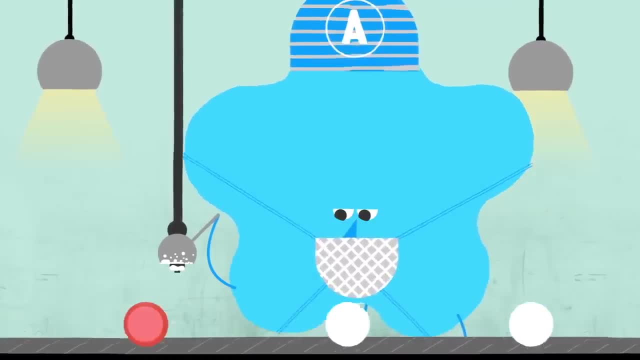 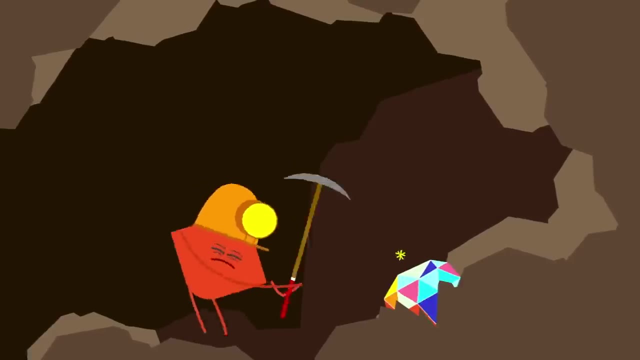 and make collagen, a kind of tissue that forms bones and teeth and heals wounds. Vitamin A helps make white blood cells key in the body's defense, helps shape bones and improves vision by keeping the cells of the eye in check. Vitamin D gathers calcium and phosphorus so we can make bones.